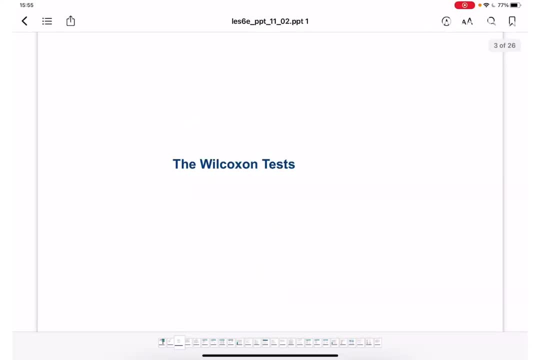 in this video I'm going to cover Wilcoxon test. Wilcoxon test is a non-parametric test which, is to remind you, it doesn't have to be from the normal distribution. there is no any requirement about distributions, can be any distribution and non-parametric test that can be used to. 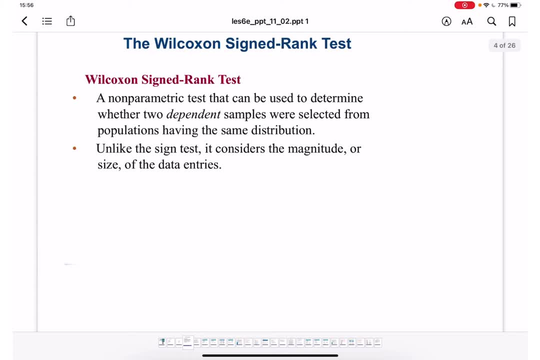 determine whether two dependent samples, two dependent samples were selected from the populations having the same distribution. that's the Wilcoxon cyan rank test. so we have two dependent samples to remind you what can be dependent. so some sample that before, in intervention and after intervention. right, so they are dependent. 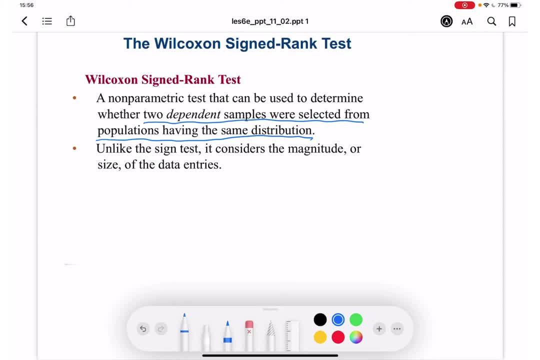 obviously, and we are going to decide, based on Wilcoxon cyan rank test, if these dependent samples were selected from the populations having the same distribution. okay, unlike the cyan test, it considered the magnitude. magnitude, just so you know, it's an absolute value. so you drop the negative sign and we use only positive absolute value, or 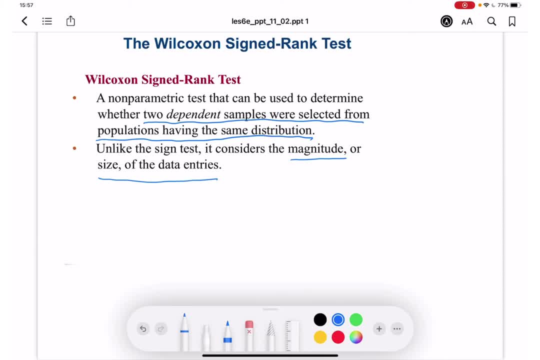 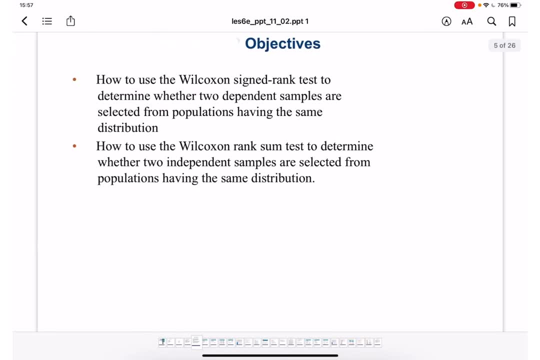 size or of any data that makes the Wilcoxon cyan rank test more powerful than just cyan test. what are our objectives here? we are going to use learn how to use Wilcoxon cyan test to determine whether two dependent samples are selected from population having same. 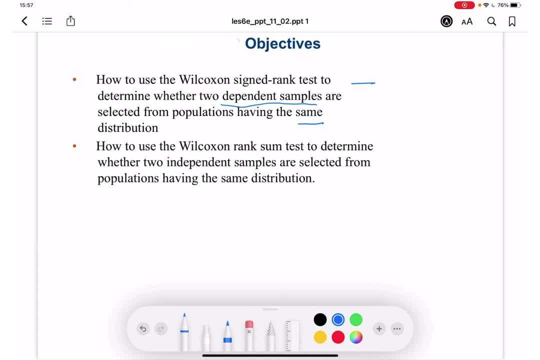 distribution. and second, we are going to find out how to use Wilcoxon run rank sum test. it's going to be next video, the second one to determine whether two independent samples are selected from population having same distribution. so Wilcoxon- um, let me see Wilcoxon cyan rank test. we are going to 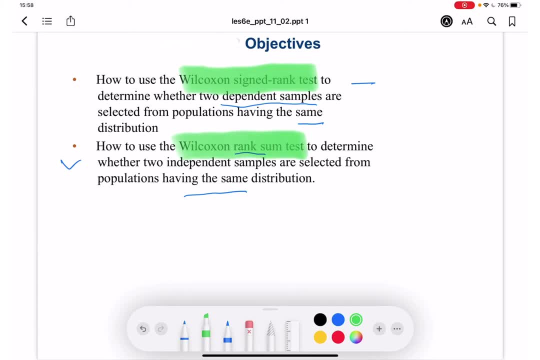 explore. in one case we are using dependent samples. in in the case of rank sum test we are using independent, but in both cases we are going to check in both cases. Wilcoxon test: it's going to identify if samples are selected from the same population having same distribution. okay, 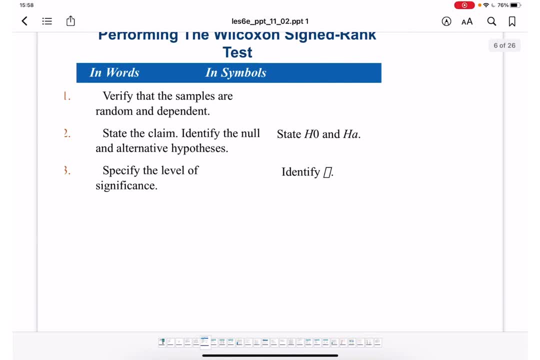 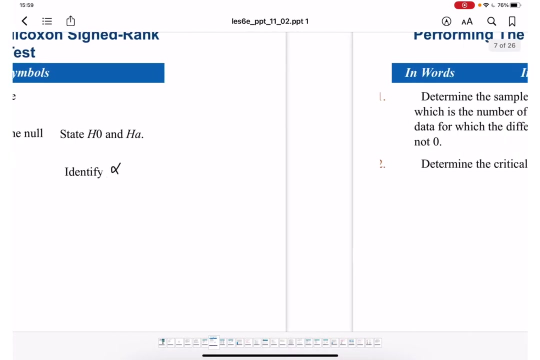 so, um, this one's, uh, those are uh, step by step, okay, so I'm not going to uh read those me clean. we need to identify. this is going to be Alpha level of significance, because I'm going to use all this on the practice, so just so you know, okay, critical value, I will. 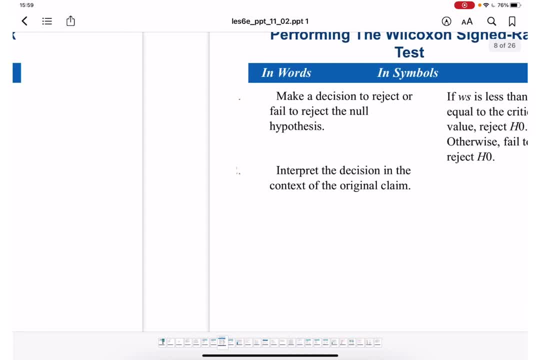 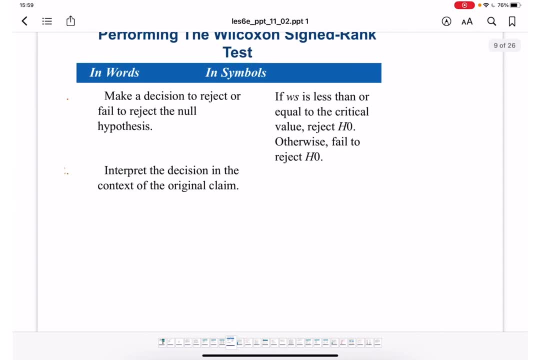 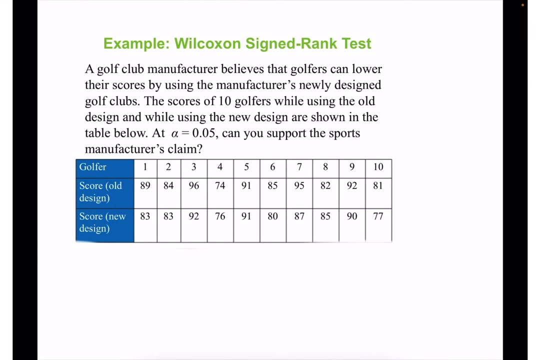 represent. so let me start. you can stop it and write down what you need here. okay, but I am moving to a practicing problem so we can learn how to use perform Wilcoxon cyan rank test. okay, here we go. a golf club manufacturer believes that golfers can lower their scores by 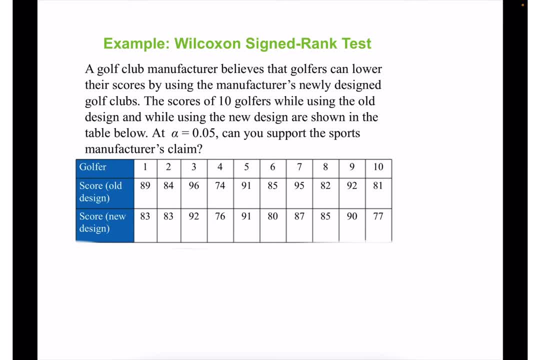 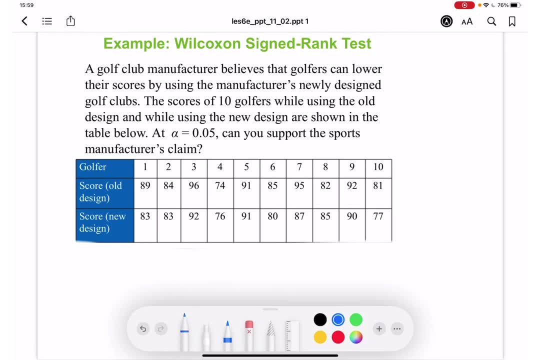 using manufacturers, a newly designed Golf Club, the score of 10 golfers. we have, uh, 10 golfers here, one, two, three, from one to ten. while using the old design- this is the old design- and while using the new design, shown in that in this table, Alpha is equal 0.05. 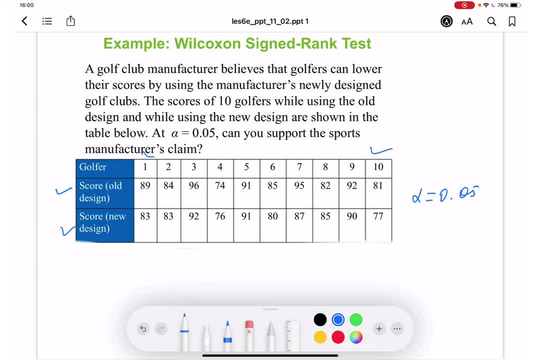 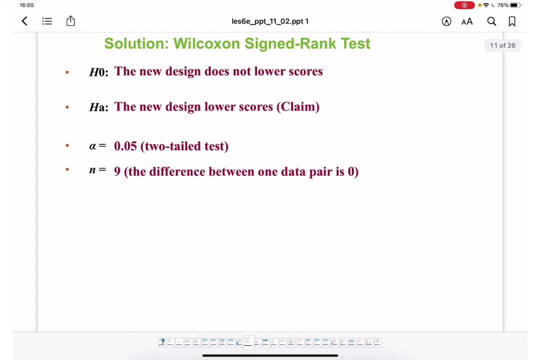 can you support the sport manufacturer's Claim that golfers can lower their scores by using manufacturer's newly designed golf clubs? So they believe in golf clubs and they believe that it can lower their scores- All right, So claim that can be lowering their scores- new design. 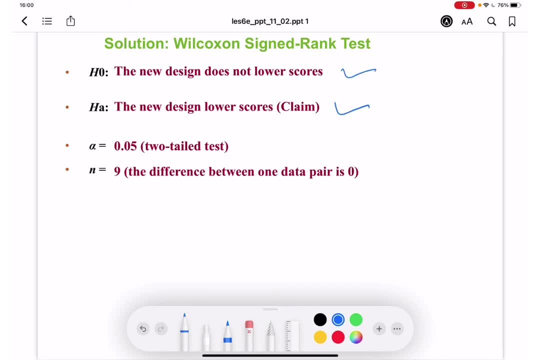 Claim null is going to be. do not lower, right. It's like equal to the old one. Okay, Since we have two-tail test, equal, not equal. alpha is equal 0.05 and n is equal 9, because we have 10, right, golfers? 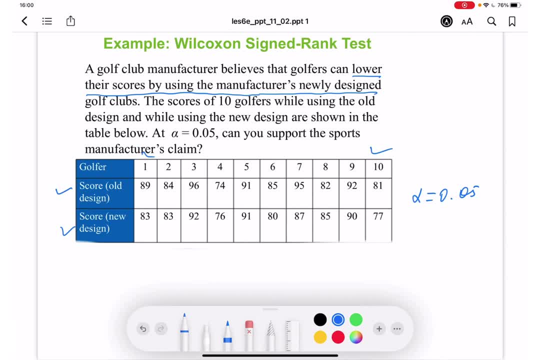 But let me see Where is it. Let me find, Ah, here number 5.. Oops, I used white color. Hold on, Okay, We have here 91, 91. So we don't count when difference is 0.. 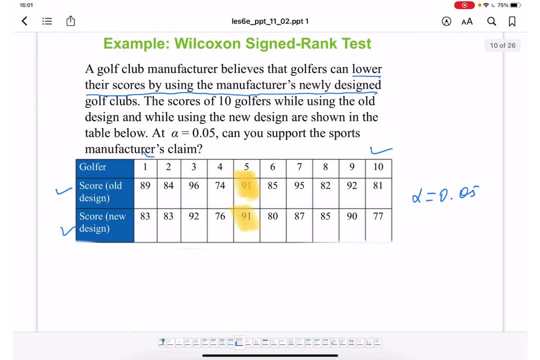 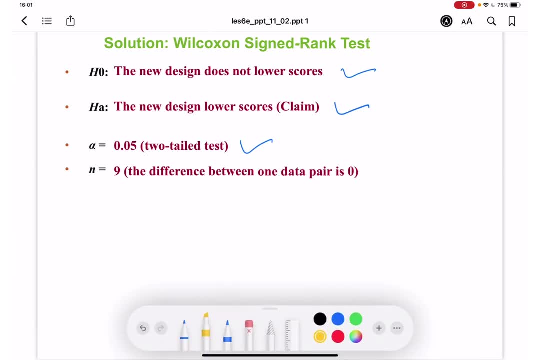 So it's identical, which means no reaction, right? Since it's the same, no reaction, then we cannot makes no sense to count it. Therefore we have here 9 instead of 10.. Make sense. At least it does make sense. 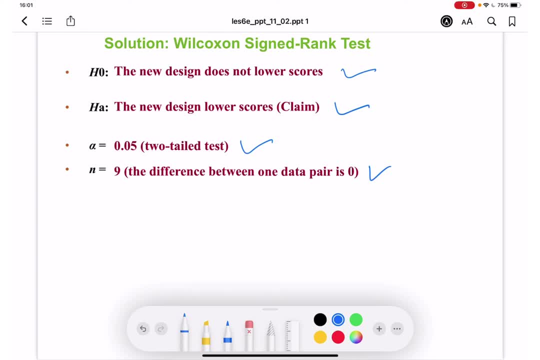 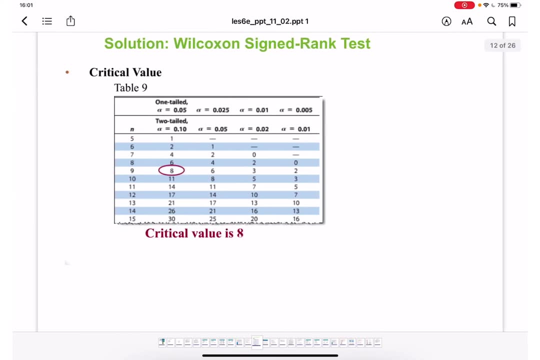 To me: Okay, Okay. So principle is same. So we are going to find test statistics, critical value, and then compare and blah, blah blah. So how we are going to get significant Wilkinson rank test? First of all to get critical value. this table you can either search on internet. 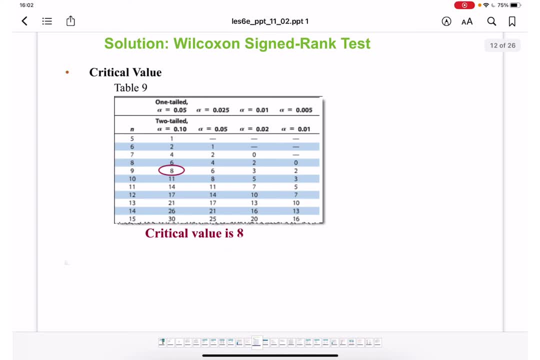 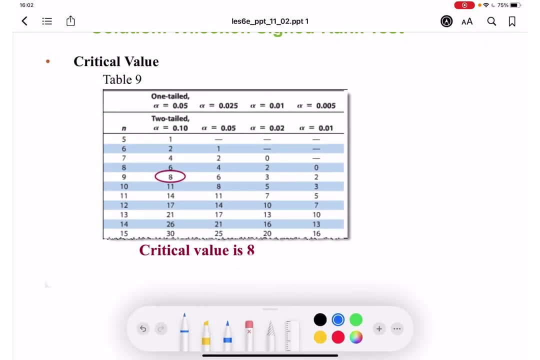 Wilkinson sign rank test, Or just to take a picture from this one. So, since we have total amount, we said we have 9, right, We eliminated 10 because there was no difference, Correct, So we have 9.. 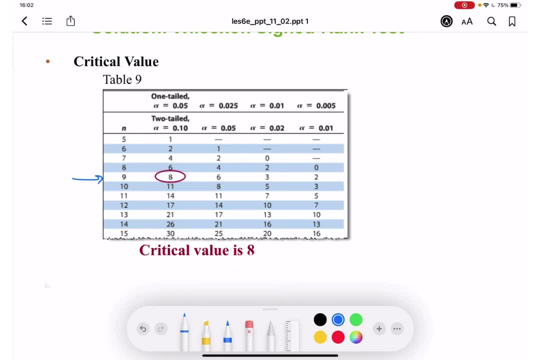 And we have one tail, is 0.05.. So, for two tail, it's going to be 0.1.. Multiply by 2, right? So we are getting, for two tail, 0.1.. And therefore our critical value, it's going to be 8.. 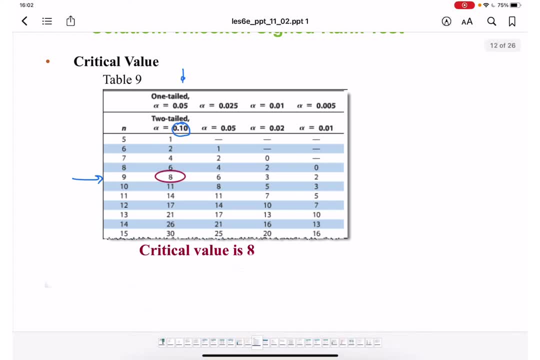 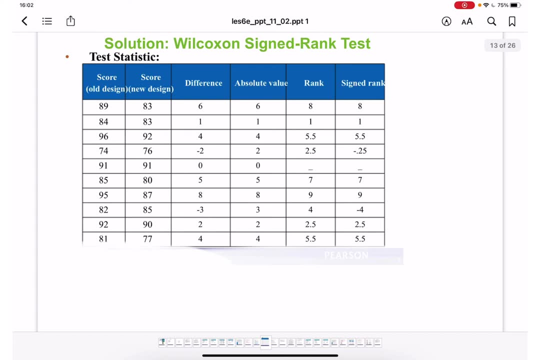 Okay, We got our critical value. Now let's find our test statistics. So how we are going to do Wilkinson sign rank test. This is all these scores from all design that you see previously in horizontal, Horizontal, Horizontal, Horizontal. 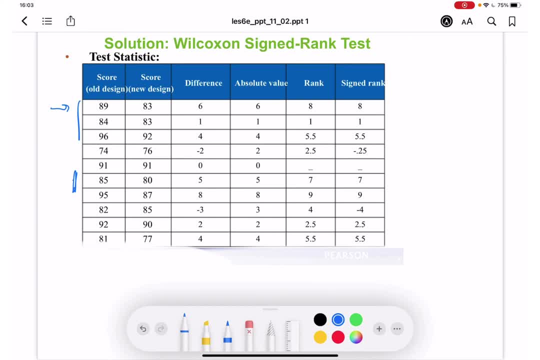 Horizontal line, now that represented in the vertical position. so score all design and new design here it is. so what we're gonna do now. we're gonna get difference between- uh, old and new designs. here is our difference. so we get here: 689 minus 83, 6, 84 minus 83, 1, and so on. okay, all the way down. 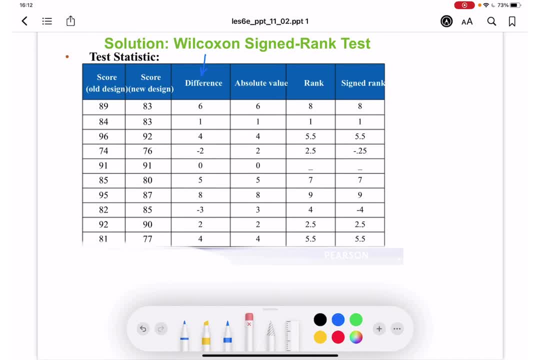 okay, next we are going to take next step. we are going to take absolute value. that's a magnitude. absolute value, which means all these negative signs. it's going to disappear. here is the negative sign disappearing. here is disappearing now. next we are going to, uh, rank them by order. what means ranks? 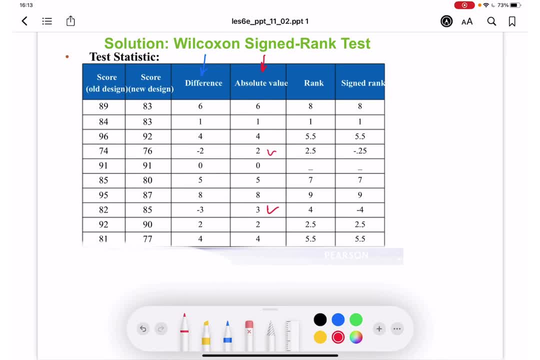 from smallest, arrange this absolute value from smallest to highest number. let's say, arrange rather like one, two, three, next it coming, let's say another three, then coming five, uh, seven, nine and so on, whatever comes. um, uh, in the order. okay, so, uh, and we are going to rank the following way: 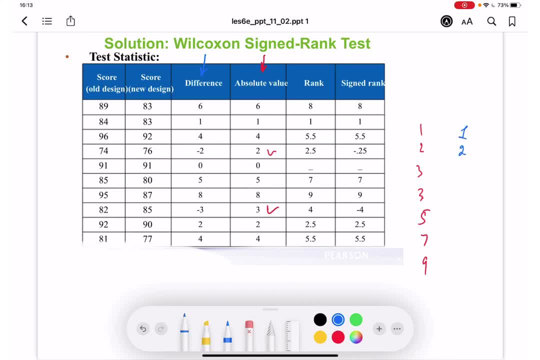 this is going to be one, this is going to be two. here i am going to have three, and since it's same three, it's three and three. so, which means that since there are both of them free, i'm going to get half of it. uh, meet, uh, halfway. two and a half. so it's going to be two and a half, two and a half. 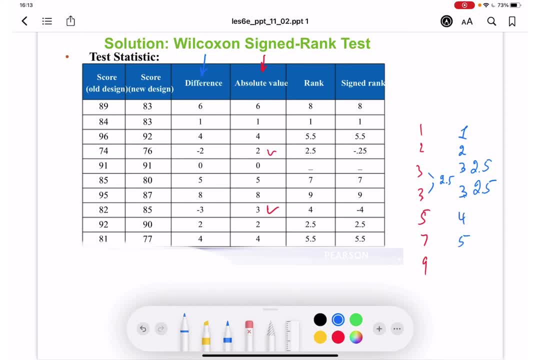 okay, and then this will be four, this will be five, this will be six, and so on. so first one is number. uh, one, first one, and then number two is coming. we have two of them, right, one and two. that's why, instead of two and three, we took the average two and a half. two and a half, yes, zero doesn't count. 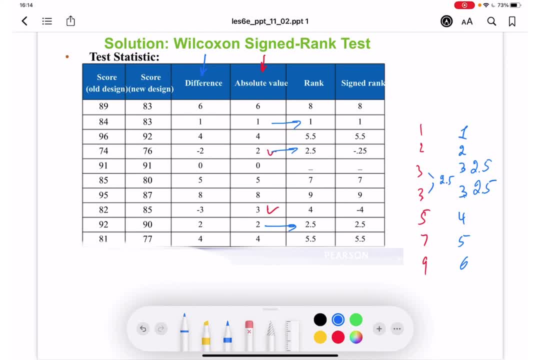 because there is no difference. and then, uh, three, we have three, it's going to be four because after three we have two and a half. so it's going to be three and a half, so it's going to be three and a three comes four. we just didn't write down three because we have two of them, we wrote down two and 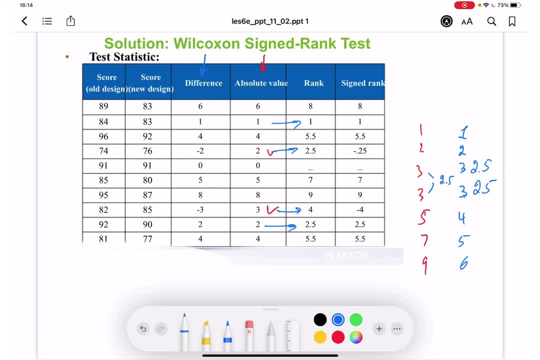 a half, two and a half, but we counted three. next is four and the fifth number, four. absolute value also looks like two of them. so instead of um, five and six, we put five and a half, five and a half, two of them. so it's the same, uh, the reason we are doing this. so we would understand that there is. 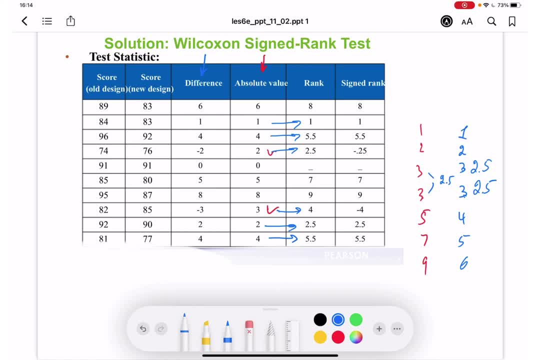 more than one of same absolute value. otherwise, if i put five and six, then you will uh accept like two different numbers, right? uh, different absolute values. that's why, okay, now let me clean this. and lastly, we are going to bring back the sign. okay, we are going to bring back the sign here, the sign rank. 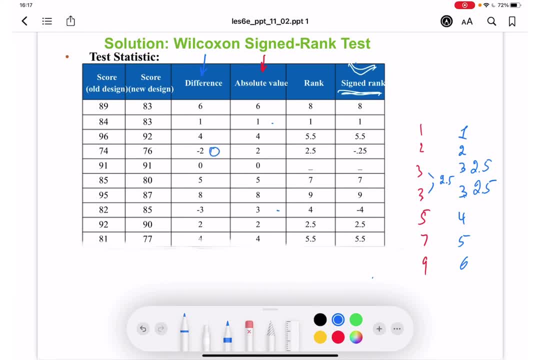 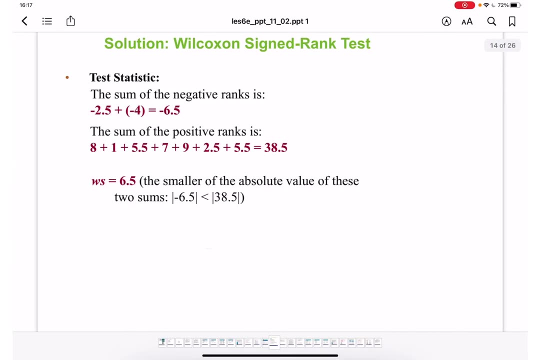 so which way means? here we had negative, so we bring back this negative, here we have negative, we bring back this negative four. what four do we need? because then we are going to do sign rank testing, meaning i'm going to add um negative. sum of negative ranks. right, we have negative two and a half and negative. 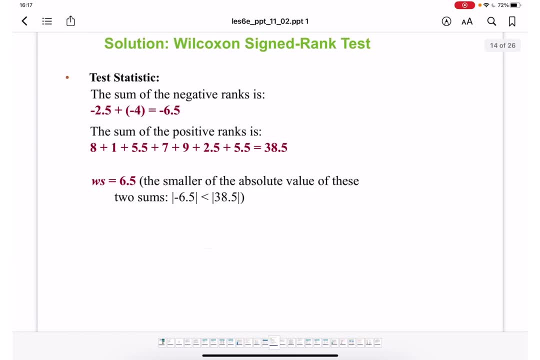 four, it will be negative six and a half. the rest we're gonna trust. eight plus one, 5.5 and blah, blah, blah. we are going to get how much we are going to get 38.5. the science, uh, rank and uh, we are going. 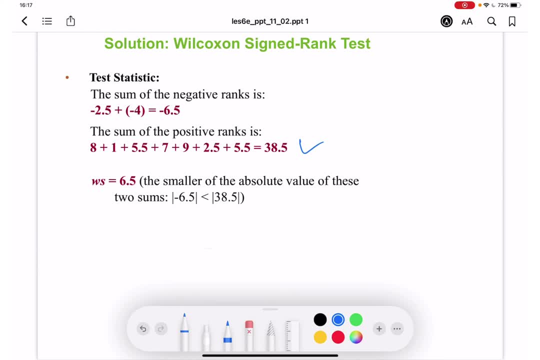 to take the smallest one by absolute value: magnitude. we are taking magnitude. it's going to be positive 6.5, and positive 6.5 compared to our critical value. that was eight. if you recall it, it was eight, remember, uh, our alpha was 0.6. 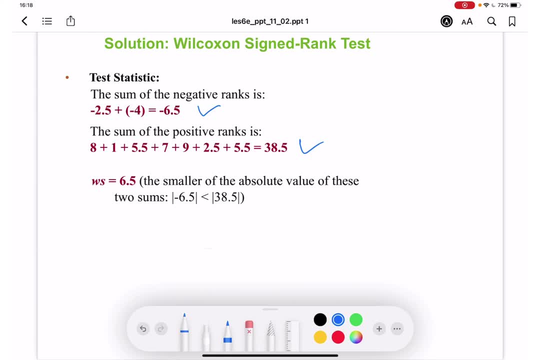 0.5. since we had to tell. we multiplied we got 0.1 and with n amount was 9. total minus total is 10. but we did minus 1 because 1 didn't give a difference between old and new design, so became 9. so critical value we got 8 and comparing to 6.5, our kind of test statistics is 6.5. 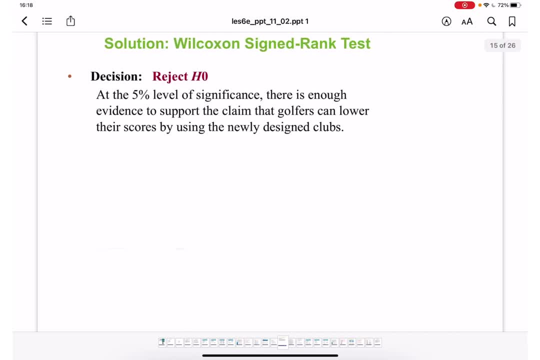 6.5 test statistics is less than our critical value. therefore, we are going to reject null hypothesis. write down: when critical value is greater than test statistics or test statistics less than critical value, we reject null hypothesis. okay, so at 5 level of significance, there is enough. since our claim is at the same time, our claim is: 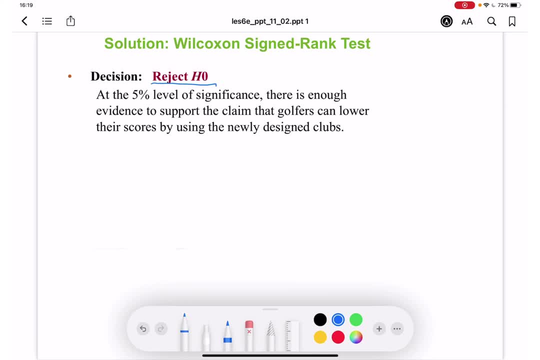 um, uh, alternative one. yes, it was alternative one. so if we reject null hypothesis, then we fail to reject alternative right and that's mean we are going, if we fail to reject, we are going to support, correct our alternative hypothesis. therefore, at five percent level, there is, uh, the enough evidence to support. 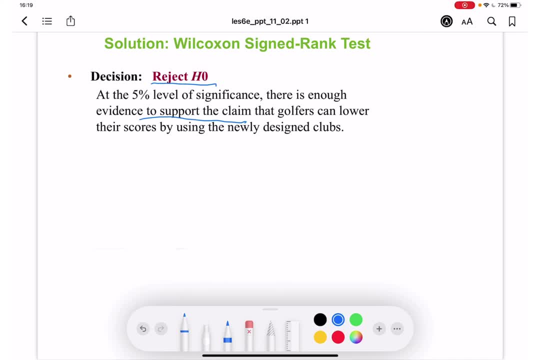 the claim that golfers can lower their scores by using a newly designed club. so you can take a note that if test statistics is less than critical value, we reject null hypothesis. if test statistics is greater than critical value, then we fail to reject null hypothesis and we dance. 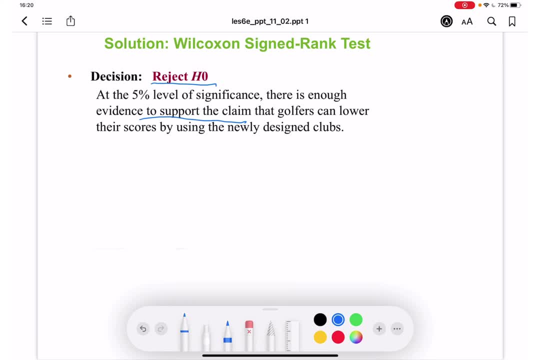 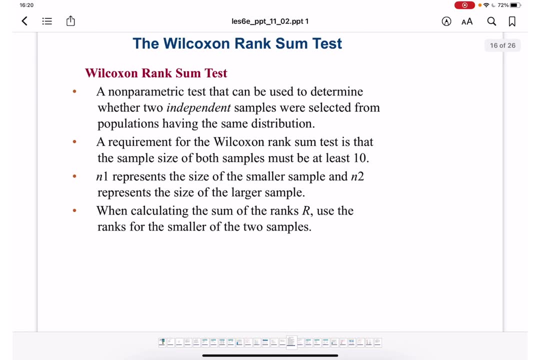 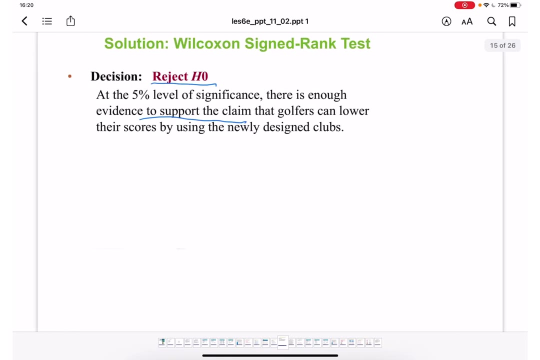 from there. this depends on what the claim is: alternative or null hypothesis? okay, rank sum. this one i will record in next video. so, um, now i'm going to turn to um assignments: record assignments after this. okay, i'm going to take a note that if test statistics is greater than critical value, we reject null hypothesis.